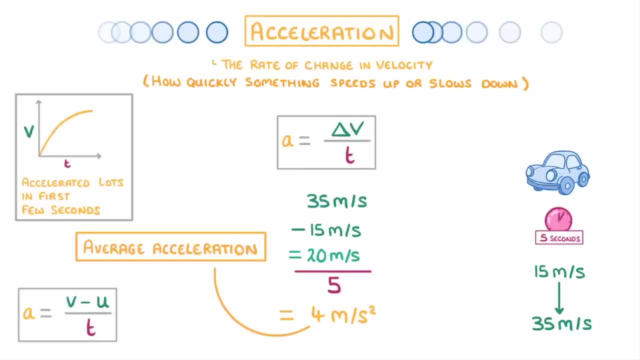 For example, it might have accelerated lots in the first few seconds, but then accelerated more slowly during the last couple of seconds. If the car had accelerated at the same rate the entire time, though, then we would call it uniform or constant acceleration. 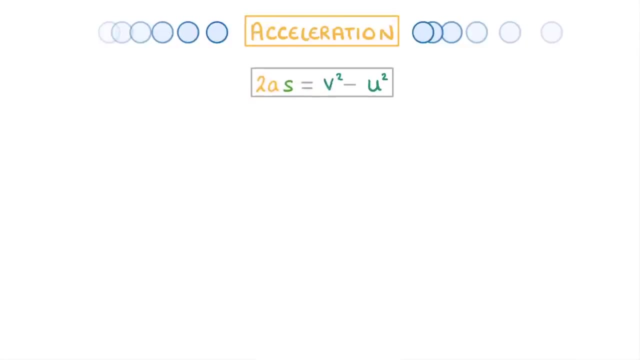 The last thing I need to cover is this second acceleration equation. We've already seen most of these letters, but now we have distance as well, which is measured in meters. If we compare this to our original equation, then we can see that the car's acceleration 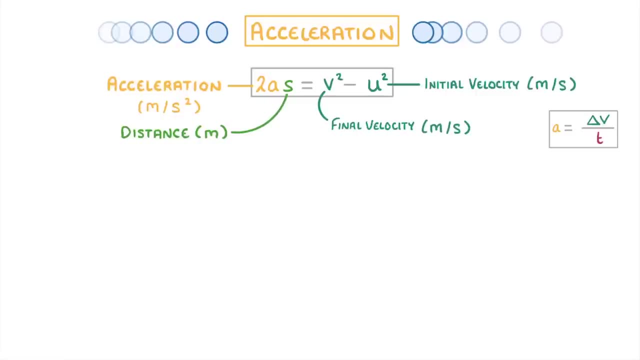 is the same as the car's acceleration. You can see that the main difference is that this new one includes distance instead of time, so you'll have to choose which of these to use, depending on the question. If you're given the unit of distance, then you need to use this one, but if you're given 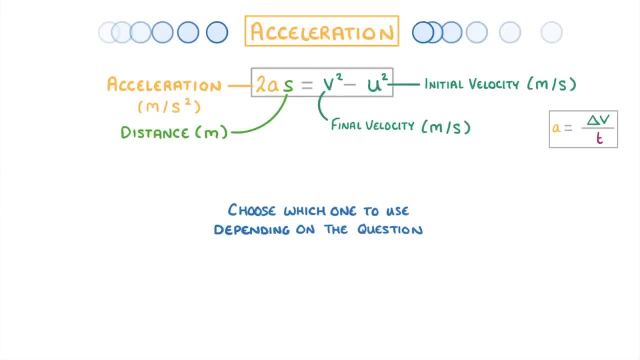 time instead, then you have to use the original one. In both cases, though, something to be aware of is that if an object starts from stationary, then its initial velocity so? u will be zero, Because it's not a constant acceleration. 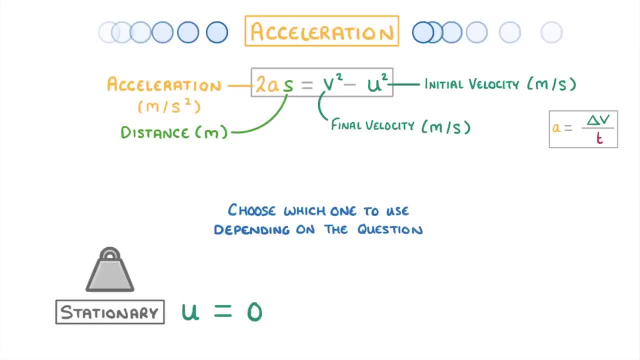 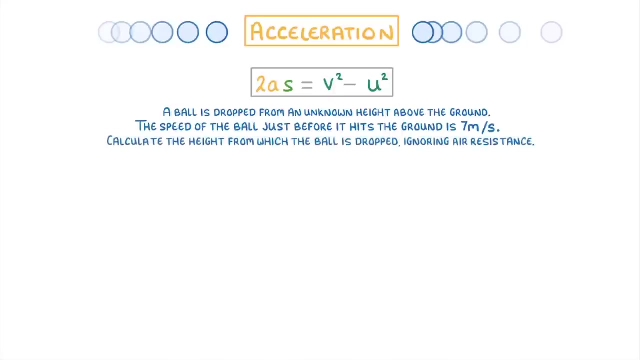 For an example, let's imagine that a ball is dropped from an unknown height above the ground. The speed of the ball just before it hits the ground is 7 meters per second. Calculate the height from which the ball is dropped, ignoring air resistance. 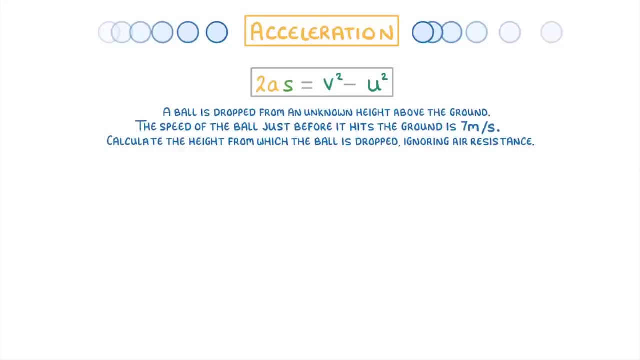 Now, at first this question seems a bit impossible, because we're only given the ball's velocity at the end of its journey, so its final velocity, which is 7 meters per second. However, because it's being dropped, we can assume that it started off stationary and 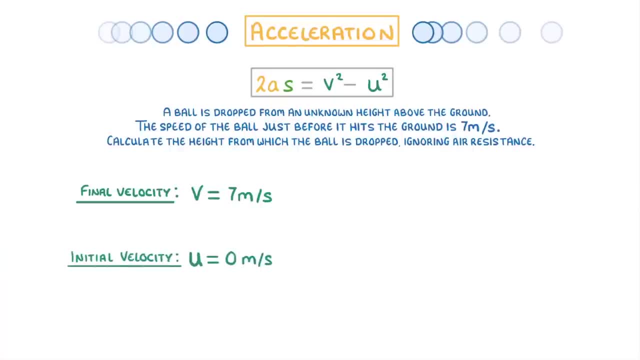 so its initial velocity was zero meters per second. Also, anything that gets dropped will accelerate downwards at 9.8 meters per second, squared, because of the force of gravity. So we now have v, u and a. To find the distance, though, which is s, we're going to have to rearrange by dividing both.